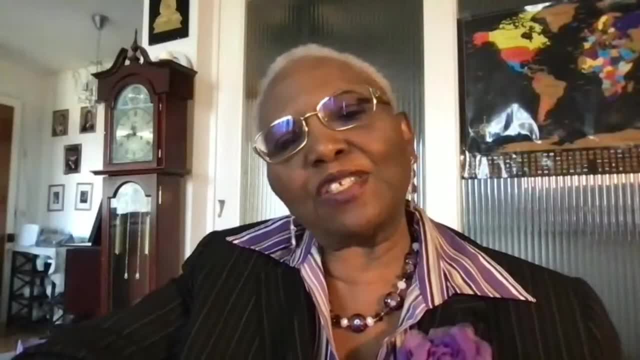 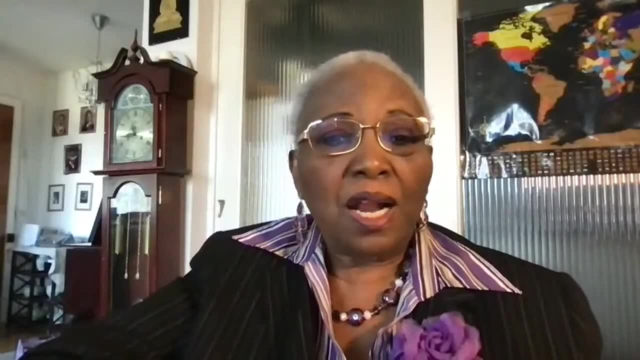 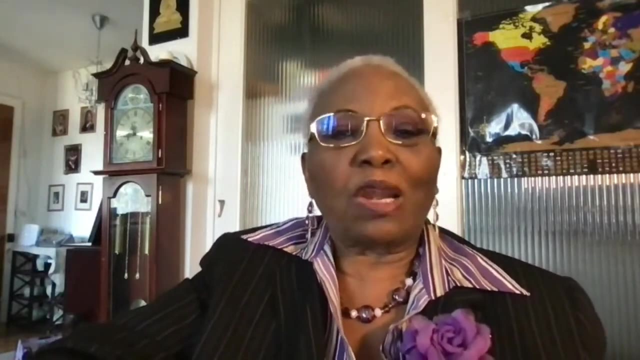 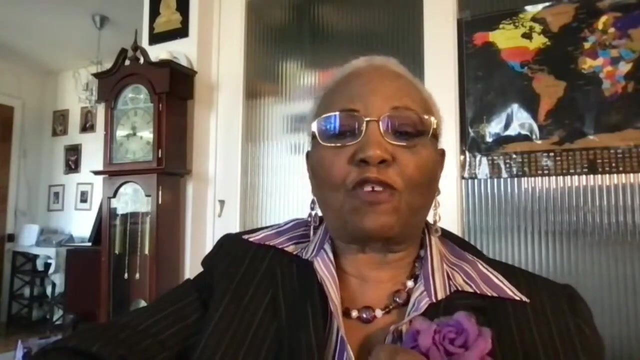 of lighting that we had when night fell. From these rudimentary means of lighting, nights were dark. I remember how I dreamt that people living outside the capital could also have access to electricity to light up after dark. As a child, I figured that these people had a right to benefit. 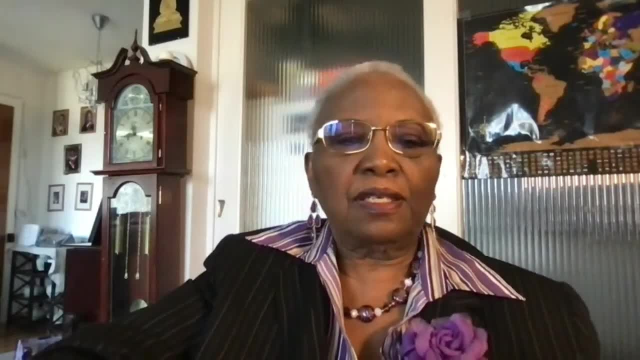 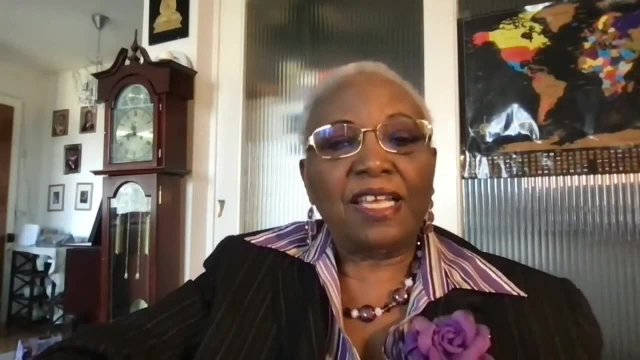 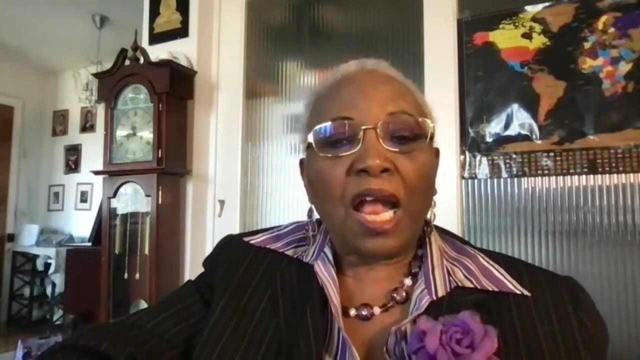 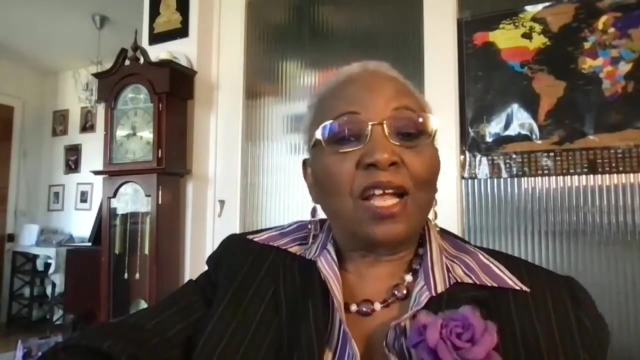 from electricity access. You see, a lot has changed since the 50s. Electricity is not just about access to light. Electricity is about access to internet, to technology, to education, to work and for health and general well-being Should access to electricity be declared a human. 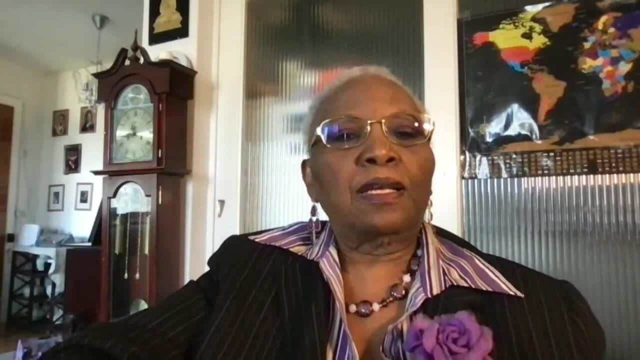 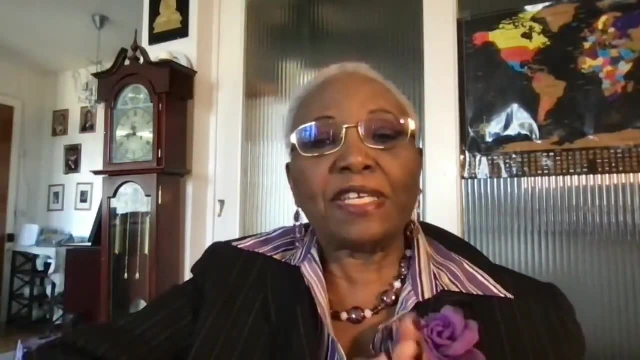 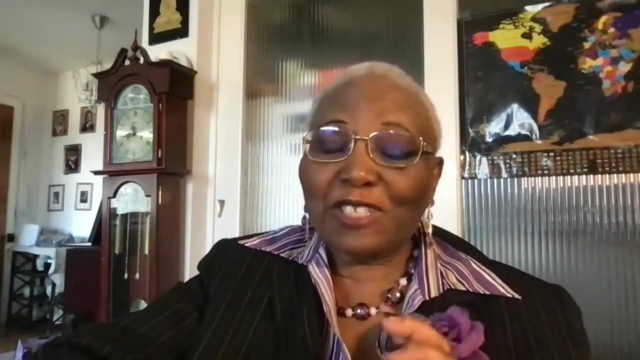 right Today, in the developed world, we cannot imagine life without electricity. A study conducted by the World Net Daily looked into the overall preparedness level of the American public. What they found is pretty troubling. Almost 50% of people who were polled said they would not be. 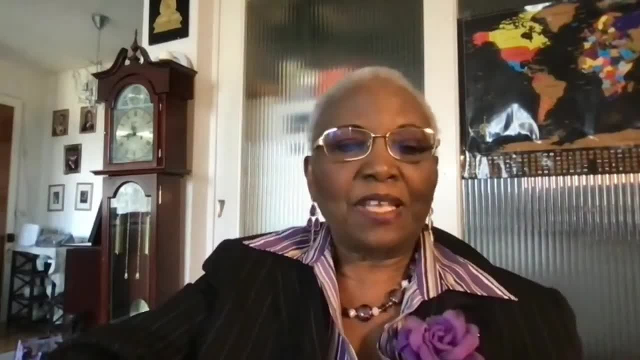 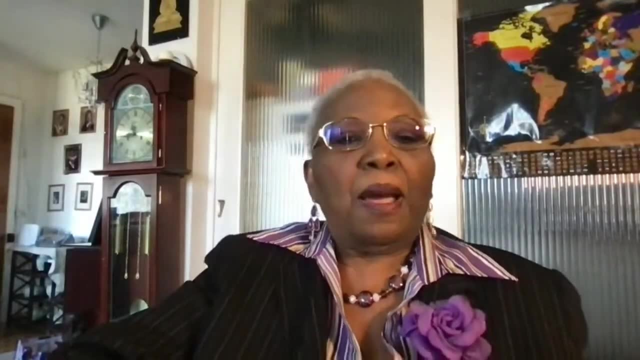 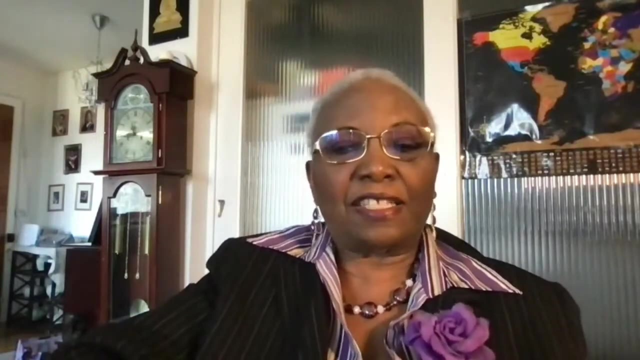 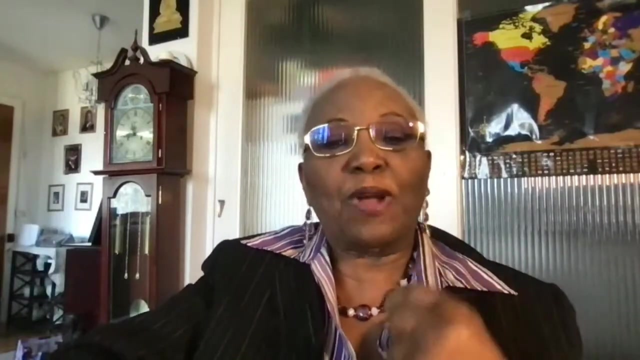 able to survive for more than two weeks without electricity. 75% of them said they would be dead within two months. Power outages in the developed countries, most recently in Texas and California, are headlines in the international press, And yet 789 million people are living without. 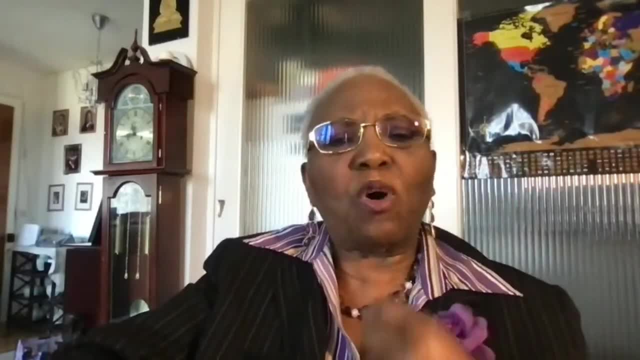 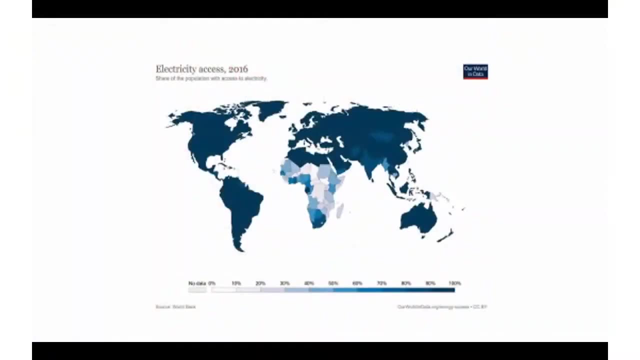 access to electricity, And hundreds of millions more only have access to very limited and unreliable electricity. Sub-Saharan Africa has the worst access to electricity, as the World Bank map shows. I have lived in both developed and developing countries and I know exactly what this means. 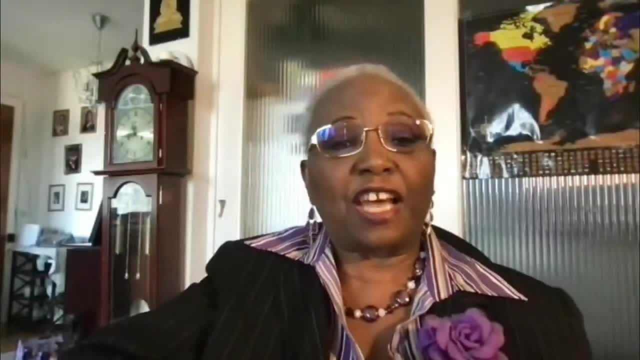 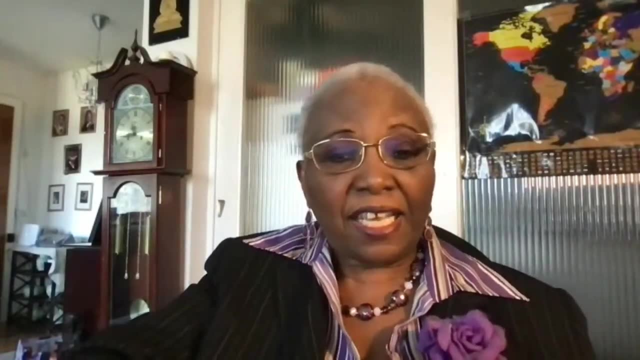 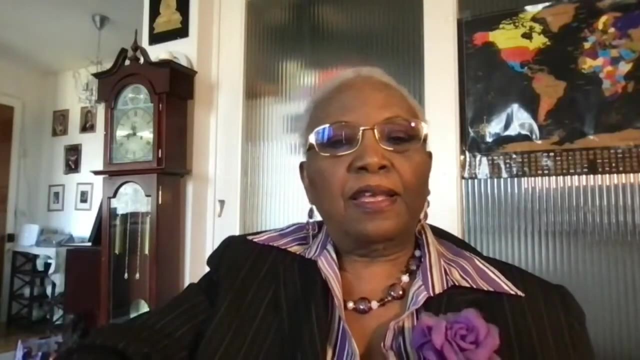 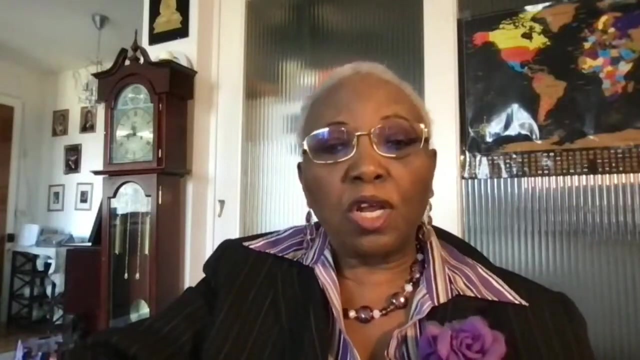 The COVID crisis has reminded us in uncertain terms of the indispensable role played by electricity today and provide insights into how the world is set to expand and evolve in the years and decades ahead. The millions of people now confined to their homes depend on electricity to work, to school, to shop. 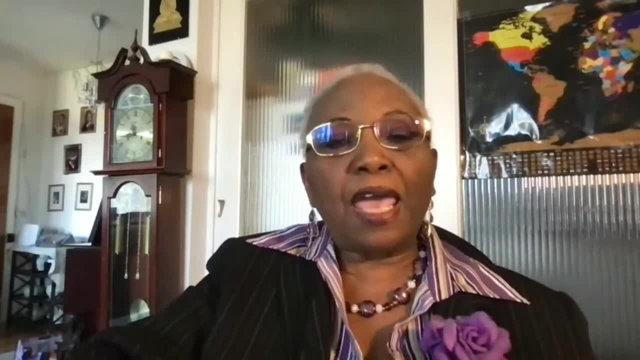 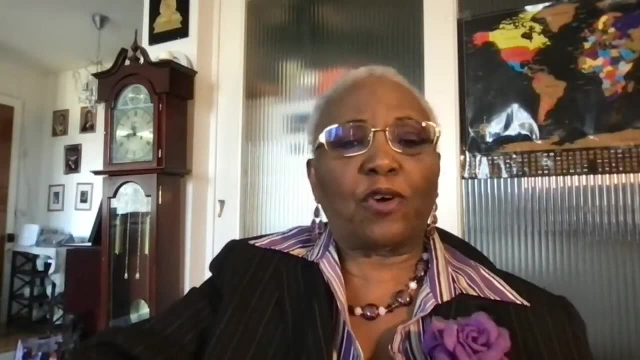 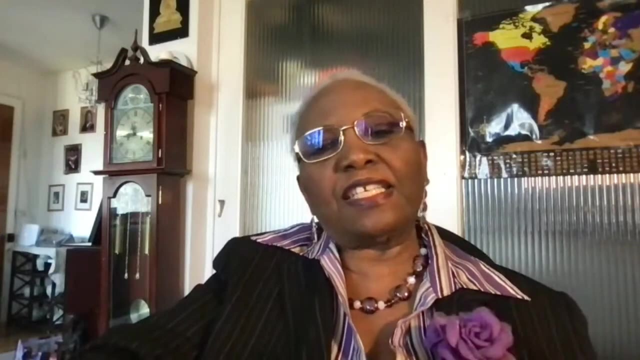 to entertain and to communicate. A reliable electricity supply is required for all of these services, as well as for powering the devices most of us take for granted, such as fridges, washing machines and light bulbs. In addition, electricity is needed for hospitals. 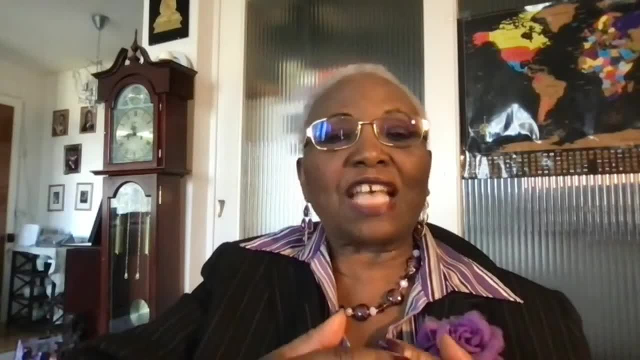 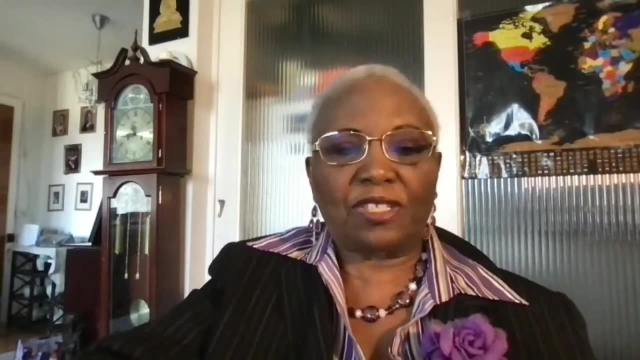 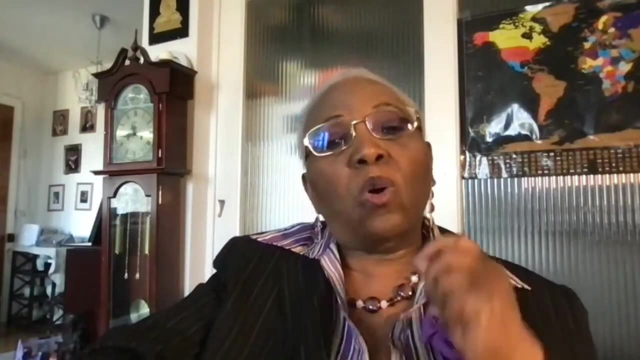 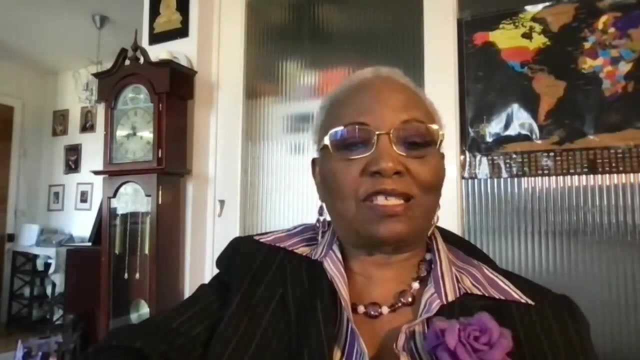 for operating medical equipment, as well as to ensure the timely communication of important information between governments and citizens and between doctors and patients. One can only imagine what this means in sub-Saharan Africa, where only an estimated 28% of health facilities have access to reliable electricity. 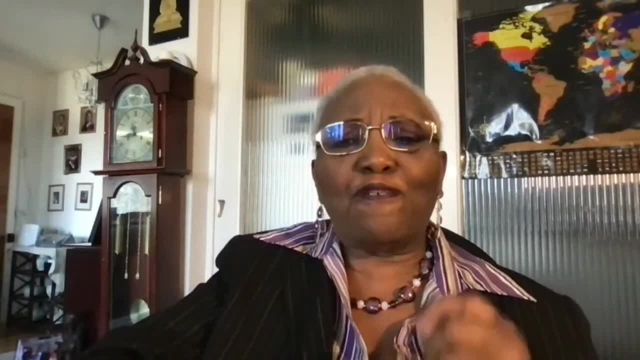 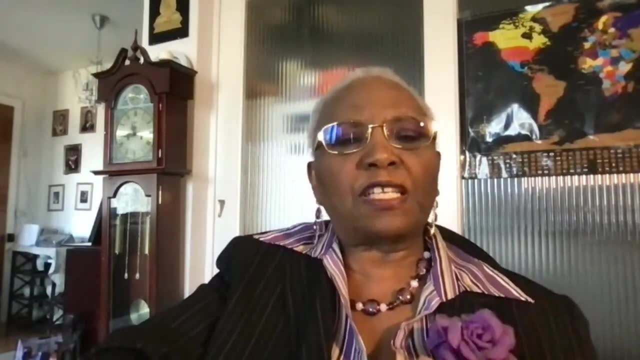 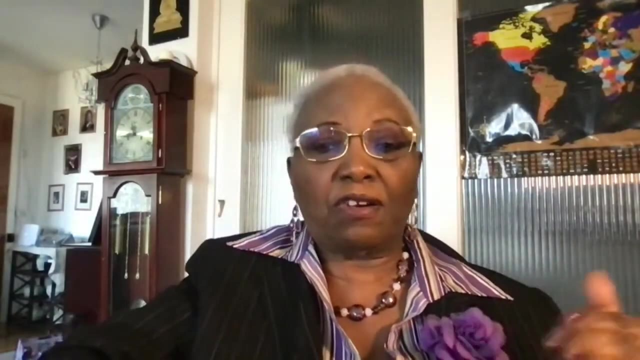 The COVID experience illustrates clearly how vital electricity is for the fulfillment of the right to work, the right to education and, most importantly, to the right to physical and mental health, as well as to the right of freedom of expression through modern technology, In some cases, even the basic human right. 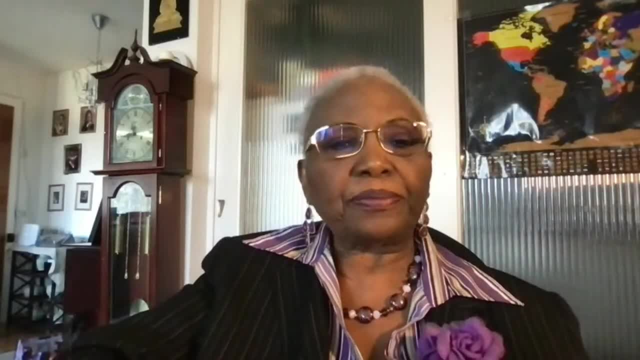 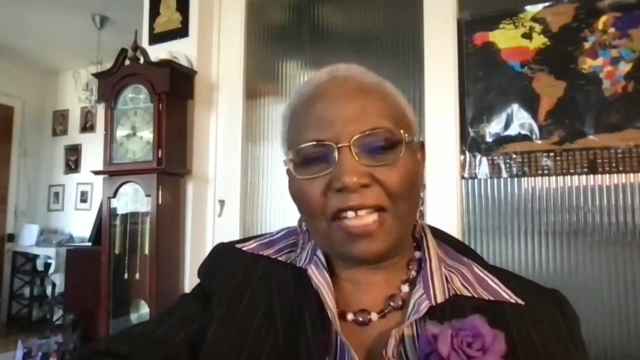 the right to life will be compromised. In the developed world, we do not even have to think about electricity access and we take it for granted. But let us for one moment think about the role of electricity access in the future. Let us stop to consider the people living. 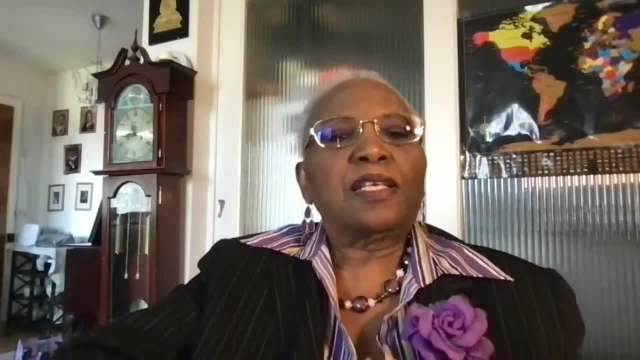 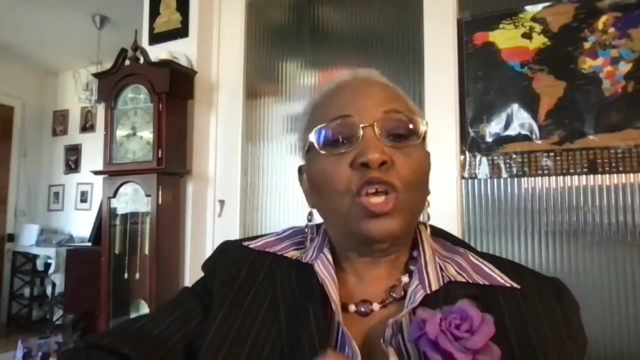 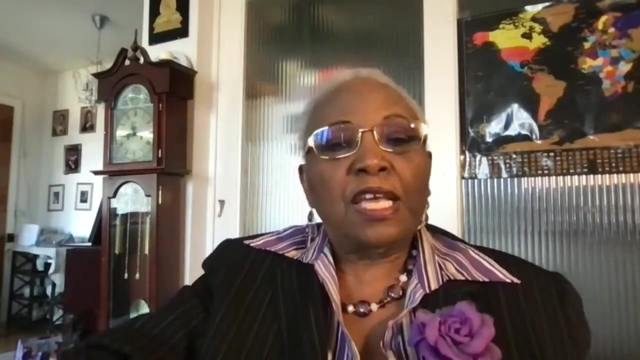 in the lighter area of the World Bank map. Steps to ensure that disadvantaged people do not have their human rights compromised during and after COVID crisis should include prioritizing electricity solutions to power, health clinics and first responders, keeping vulnerable consumers connected and increasingly reliable uninterrupted. 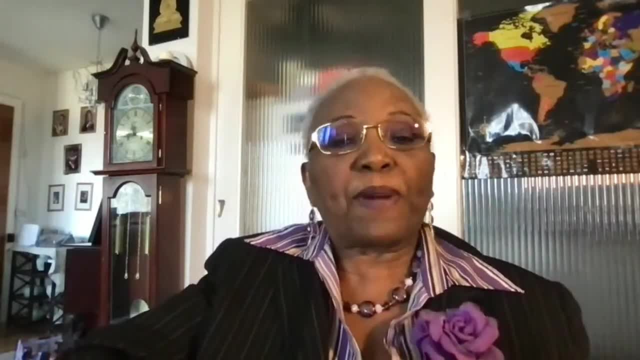 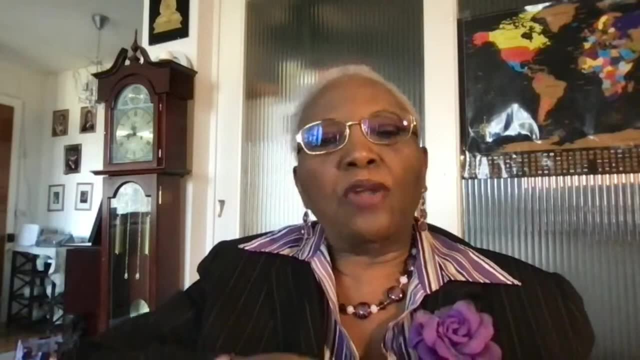 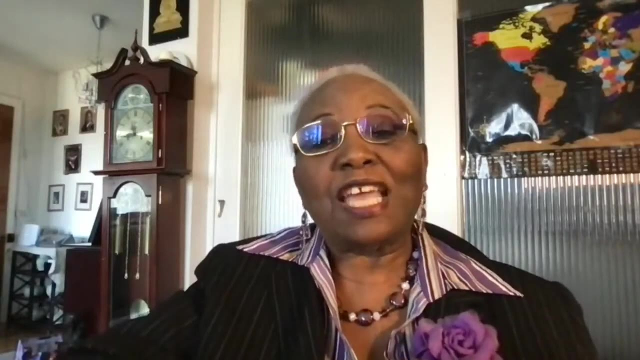 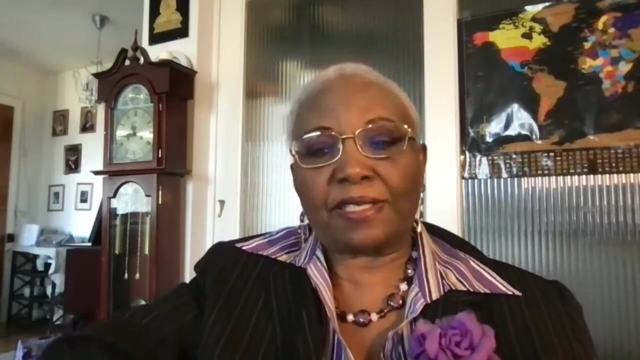 and sufficient electricity production in preparation for a more sustained economic recovery. Simply put, under the prevailing situation that exists in the world today, the denial of access to electricity is a human rights abuse. Something needs to be done, and fast. The United Nations has well established human rights. 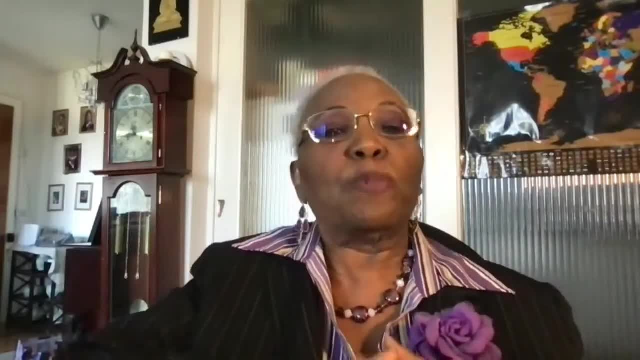 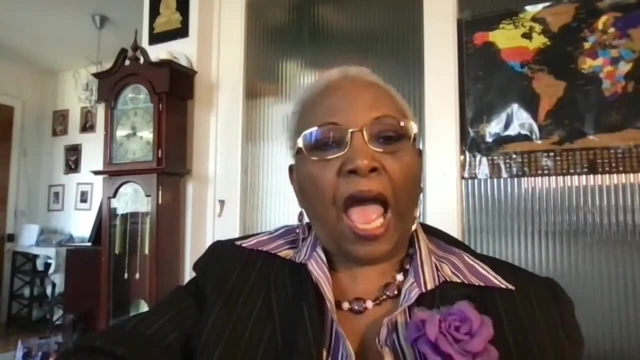 many of which are contained in the United Nations Act, Many of which are contained in the Universal Declaration of Human Rights, which was adopted by the United Nations General Assembly in 1948, and in the two covenants of civil, political, economic. 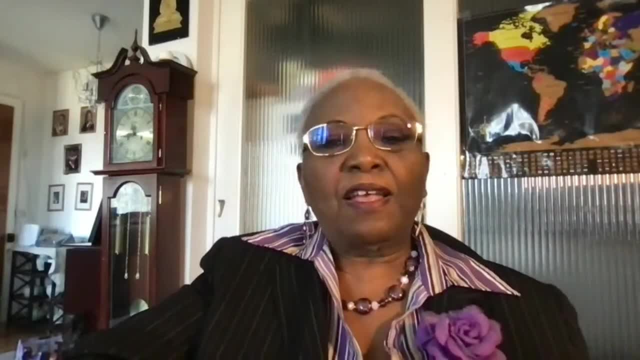 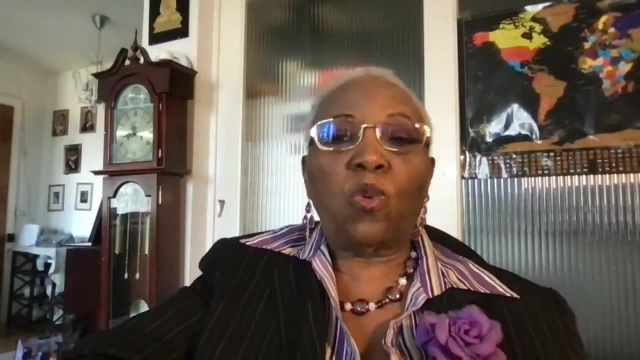 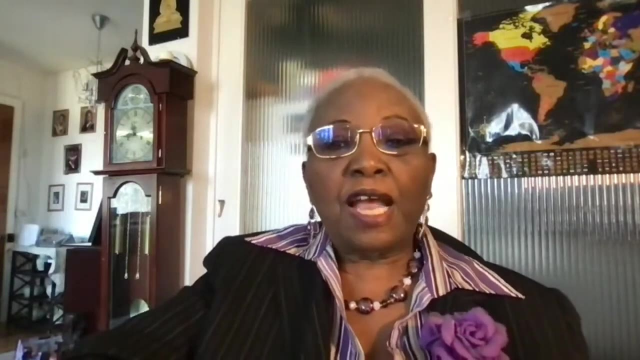 social and cultural rights of 1966. These rights include, inter alia, the rights to life, freedom of expression, health, food, water, housing, cultural development, property and home and privacy. Thank you, The United Nations has long been the держaver. 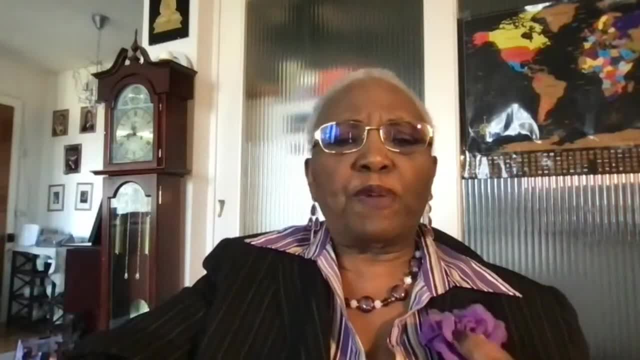 of a. secondly, changing the public's view of the world and the internal relations of society and society as a whole. This is why I think it's important to remember that the world is changing and that the world as a whole has changed since the 19th century. 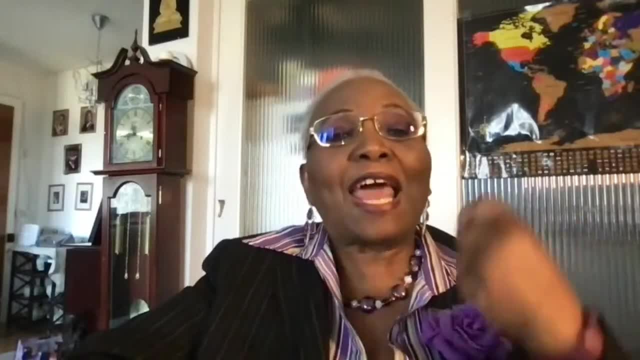 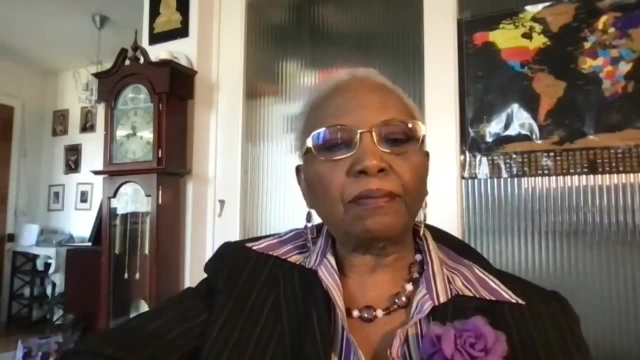 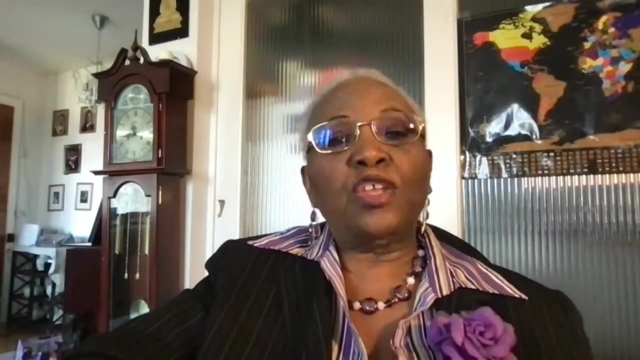 But the world has changed since And human rights need to be viewed in the light of current realities. We need to think outside the box. Throughout my career at the United Nations, I have promoted access to electricity in humanitarian situations and in development activities. 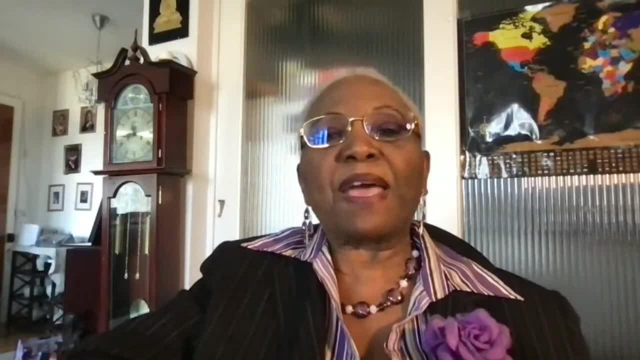 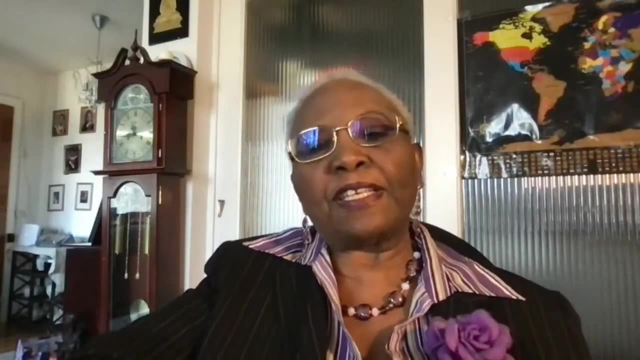 I have become the leader of the United Nations Tribunal in America and I will continue to do so in the future. to represent my country, Sierra Leone, for six years at the Human Rights Council. At the Human Rights Council, I participated in the reviews of the human rights situation. 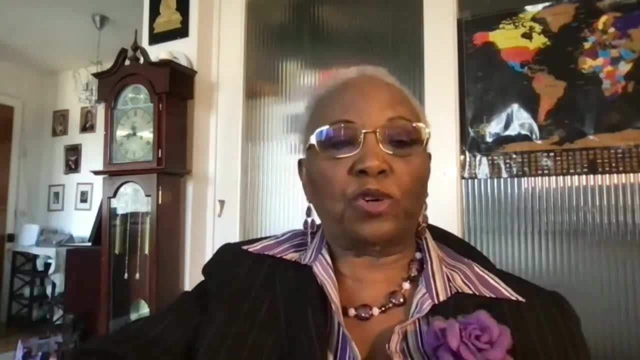 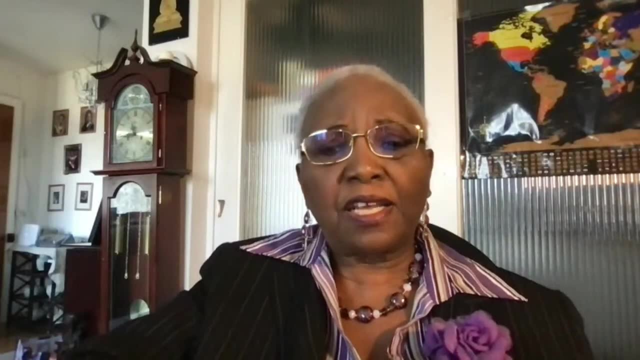 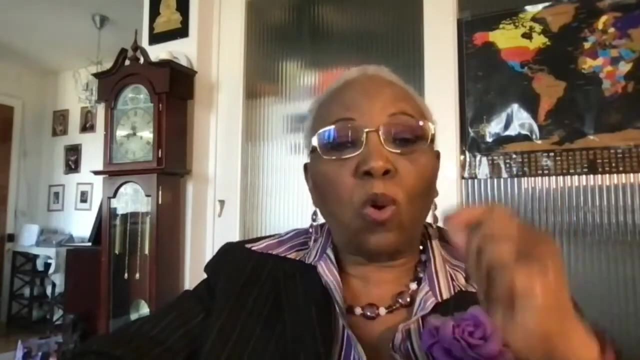 in over 90 countries from all over the world. From these reviews, one could see clearly that the countries that have failed in making progress towards the realization of the economic and social rights of the other peoples were countries with low access to electricity. In addition, 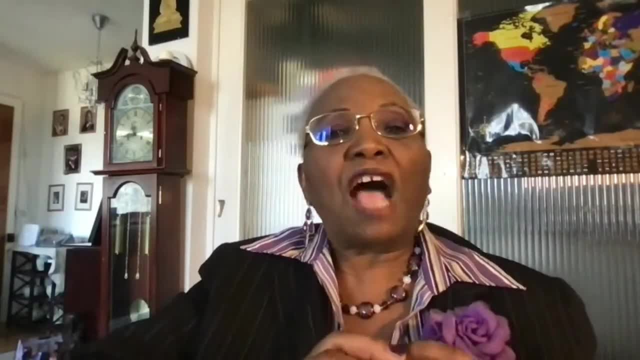 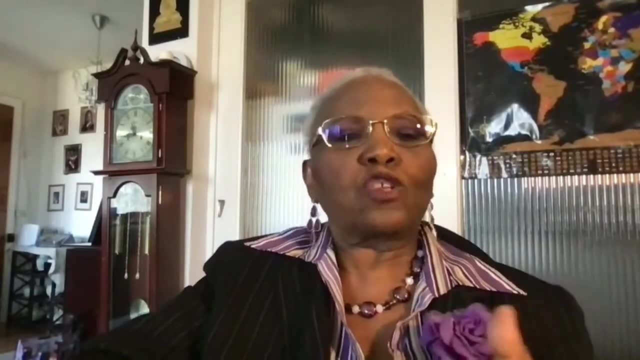 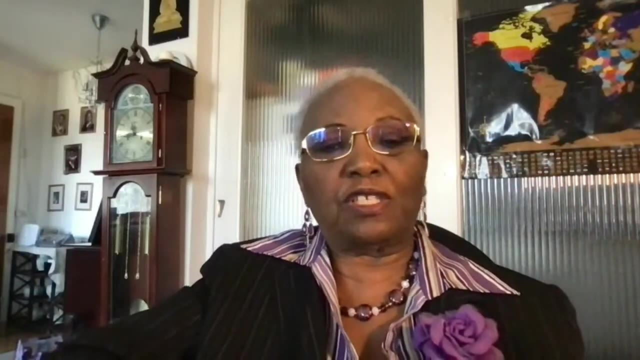 given the fact that developments in technology have made it possible to address even the political and civil rights through the use of electricity supply, for instance to power mobile communications, the full realization of these rights will also be found wanting without access to electricity After my retirement. 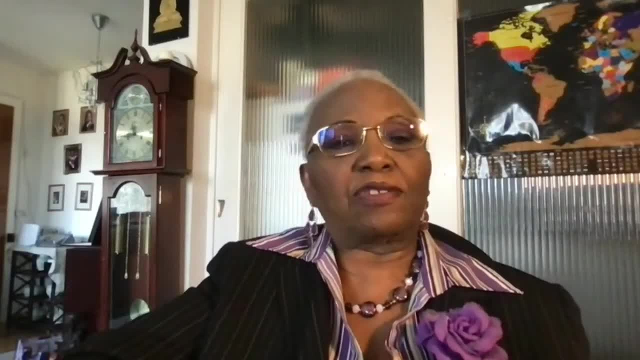 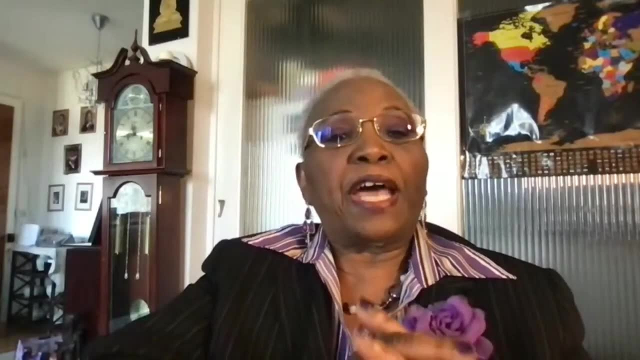 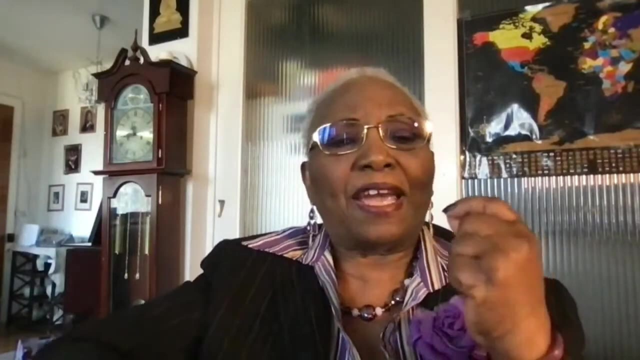 I was appointed by the Human Rights Council to lead a team to hold consultations and advise the council on steps to take to enhance its role in preventing human rights violations. One of our recommendations is that the council needs to pay greater attention to the implementation of recommendations made to member states in countries of use. 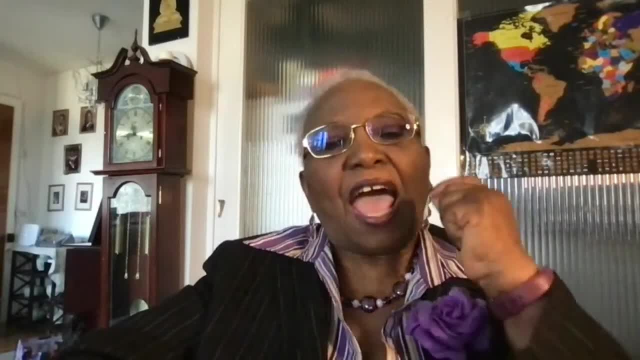 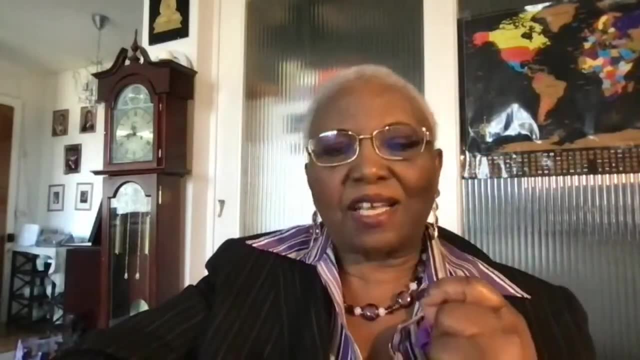 When this is done, it will be evident that access to electricity is a major risk factor for the development of human rights. This is a key to prevent human rights violations, reason why human rights are being violated and that the council has a role to play in. 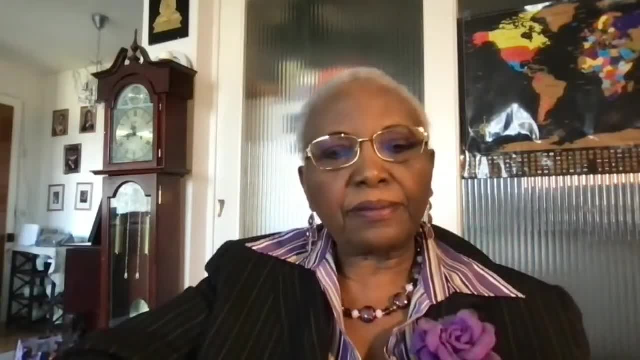 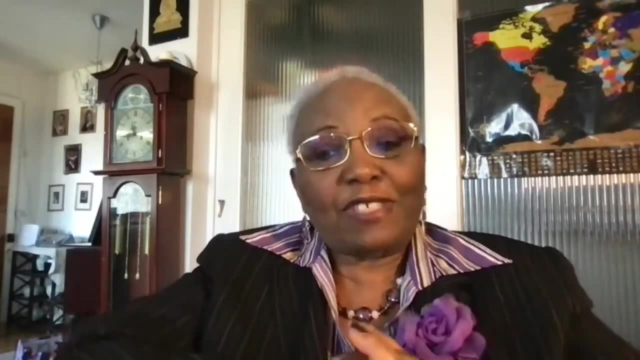 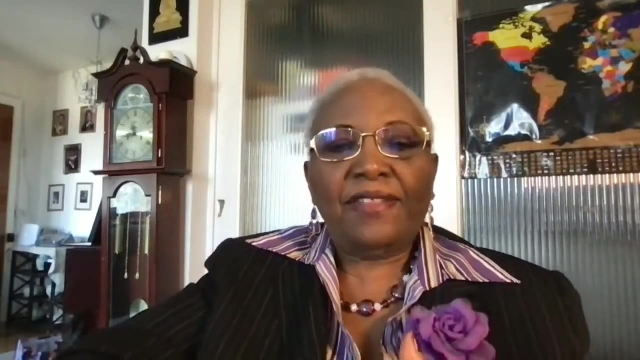 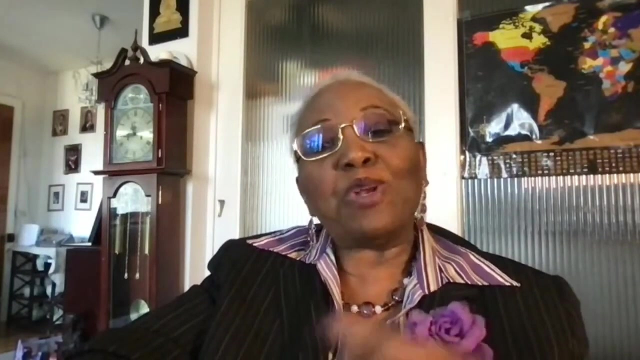 ensuring that such access is not denied. From the foregoing, it is clear to me that access to electricity is an overarching human right, And yet there are solutions to provide electricity to the most remote corners of the world. and to illustrate this, I will go back to where I started. 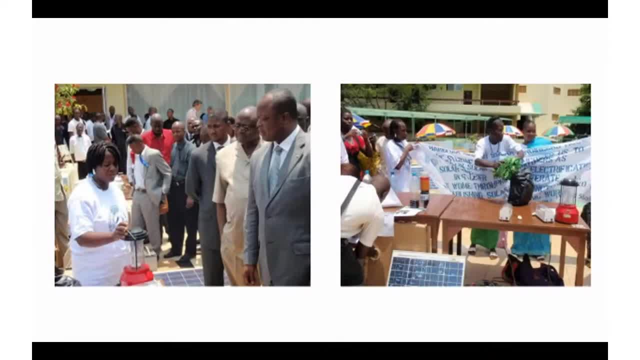 This is a solar lantern being mass-produced in Sierra Leone by illiterate women who are trained to produce solar lanterns for use in remote areas with no access to grid electricity. This is to show the potential of renewable energy to provide much-needed solutions. Indeed when I worked as energy policy advisor in Sierra Leone, I initiated solar energy. 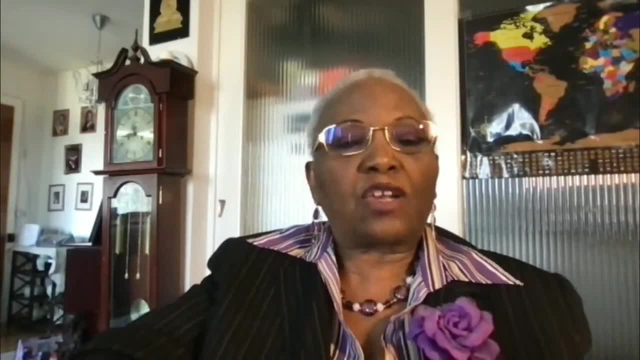 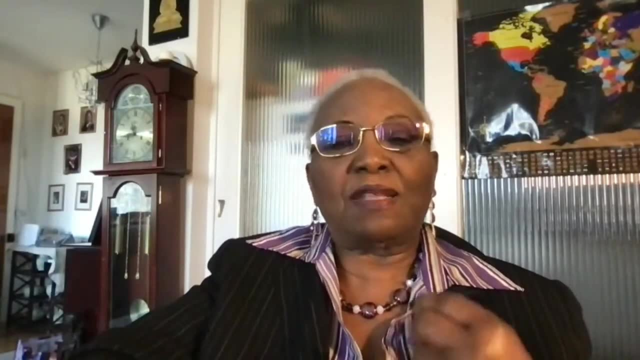 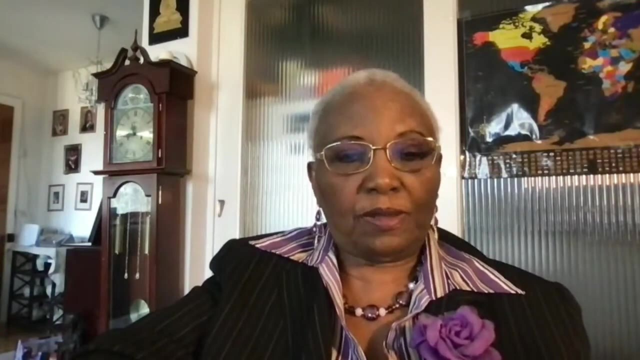 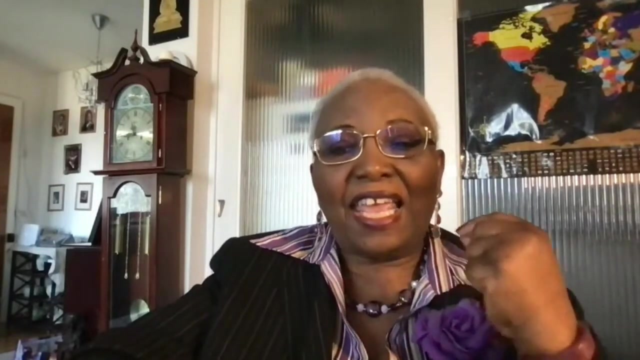 solutions to power health clinics, Schools and community centers in remote areas, as well as the installation of solar streetlights to provide security in the major towns and cities at night. But progress has been slow, even in my own country. What is needed to accelerate access is declaring electricity as a human right and making governments 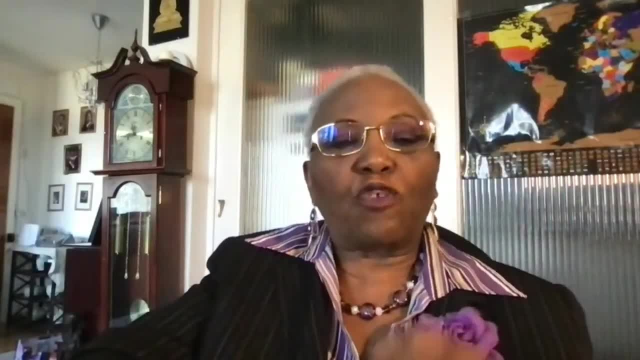 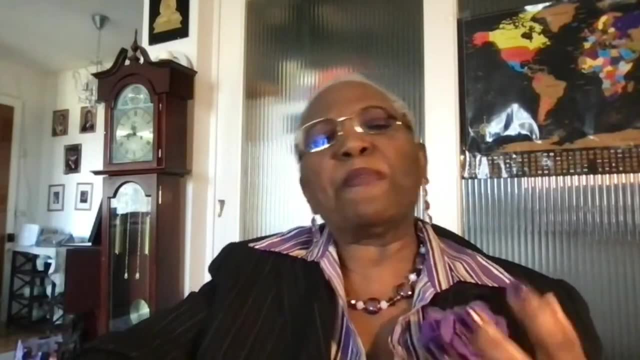 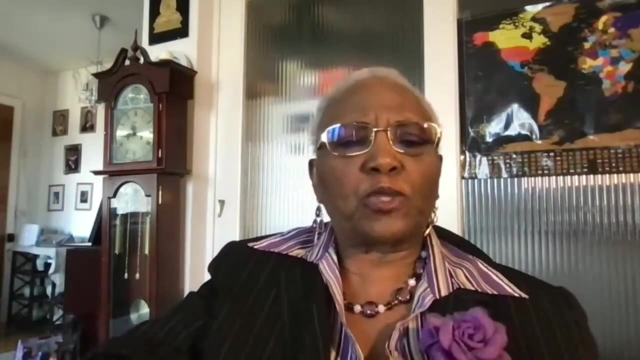 responsible and accountable for the lack of comprehensive electricity. We need to make efforts to ensure such access. Some people have expressed concern that access to electricity to meet the needs of all would lead to greater use of fossil fuels, with the potential to increase emissions of carbon. 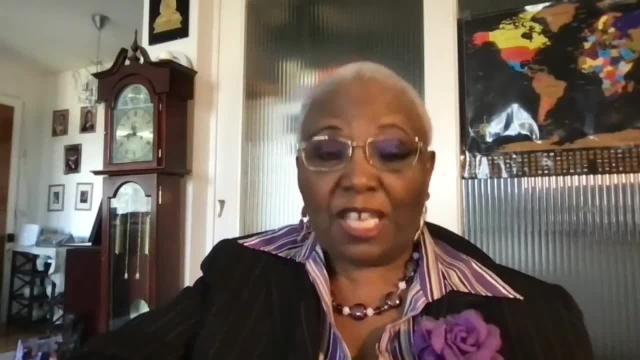 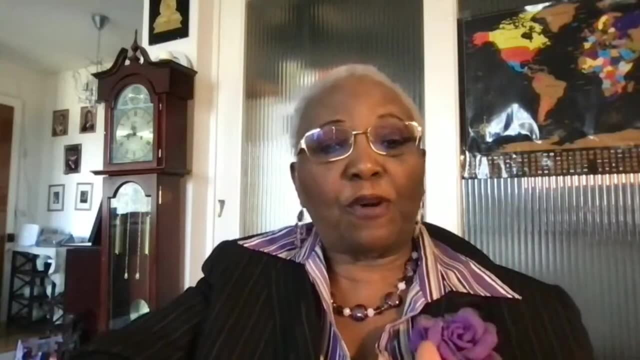 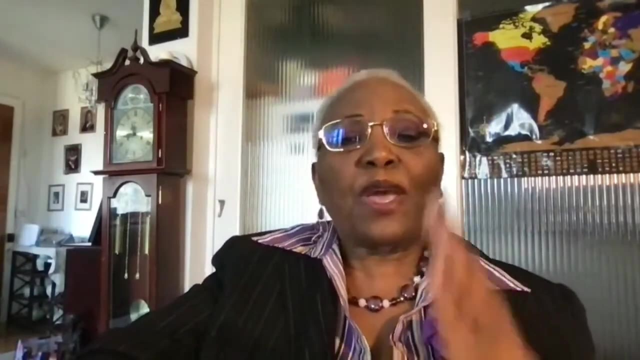 dioxide and pollution. I find this argument hypocritical if it is made by those who consider themselves champions of human rights and who benefit from access to electricity in their own countries. Yes, I agree. Yes, we need to maintain a safe environment, But we also need to ensure that the rights of all are respected. 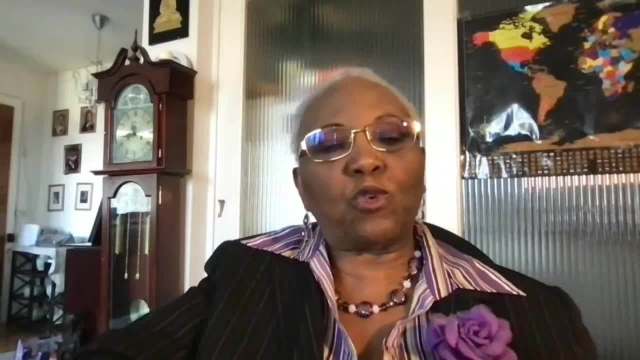 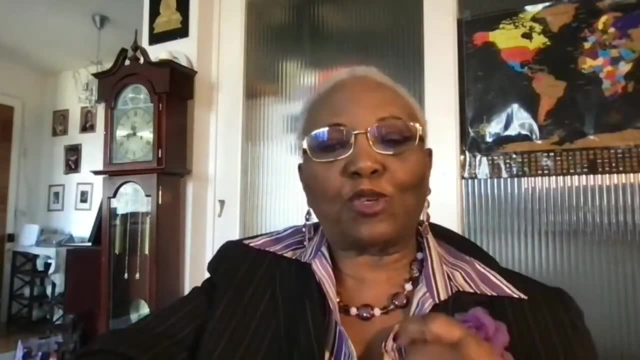 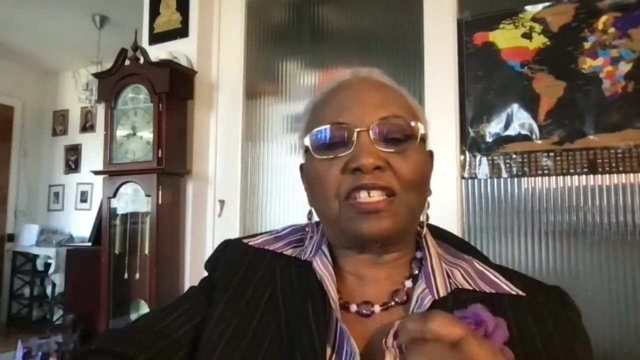 The response should therefore be to promote electricity production by using renewables. This would involve intensifying research that would lower the cost of electricity production from renewable sources and providing assistance to poor countries to exploit the renewable energy sources that are available to them, And I think this is a very important point. 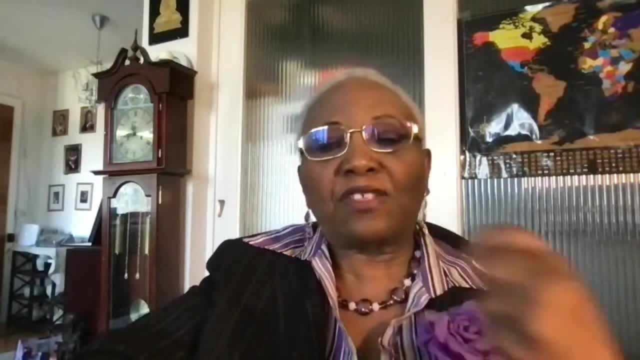 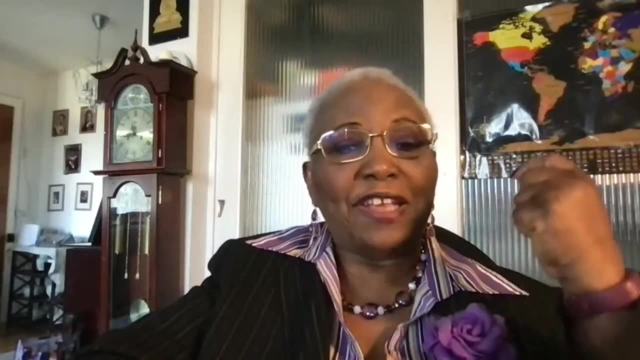 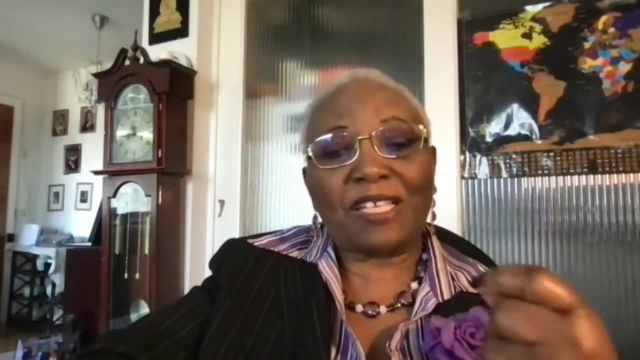 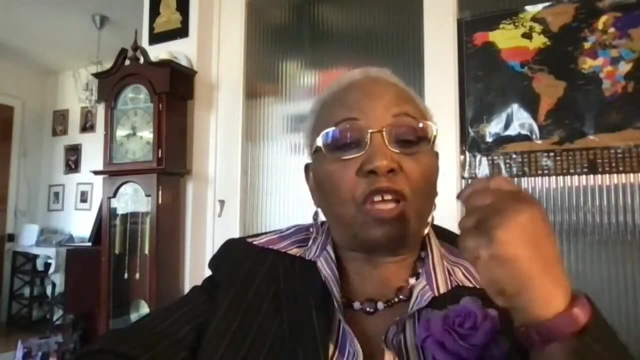 electricity access, But implementation of such plan is moving at a snail's pace. Meanwhile, poor people will continue to suffer and some will even lose their lives due to lack of electricity access. The whole problem is in how far we can go. 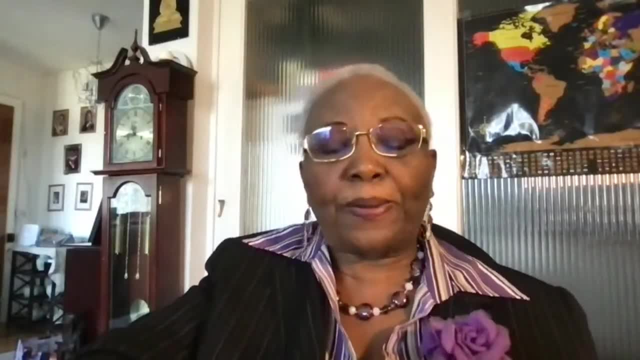 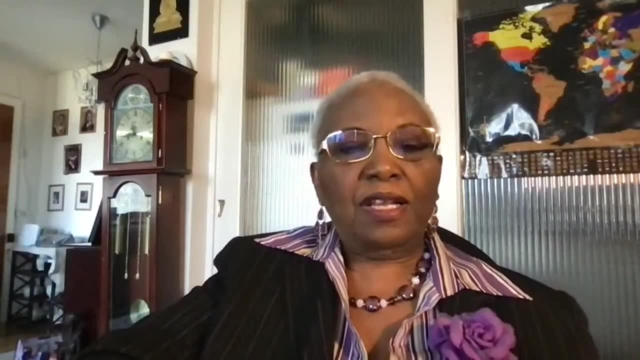 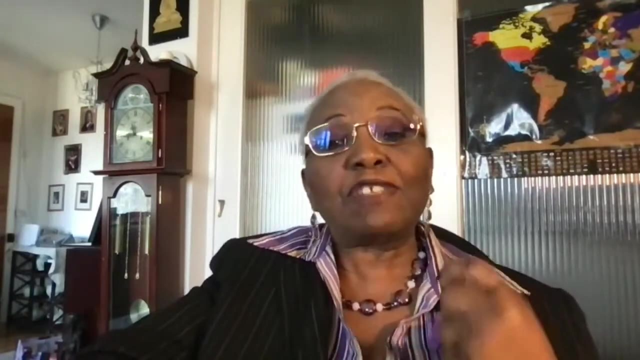 The whole problem is in how far we can go. The whole world should be concerned about this. So what do I think should happen now? Let me start by saying that there had been a general reluctance to bring energy in general, and electricity in particular, into the debate at the United Nations. 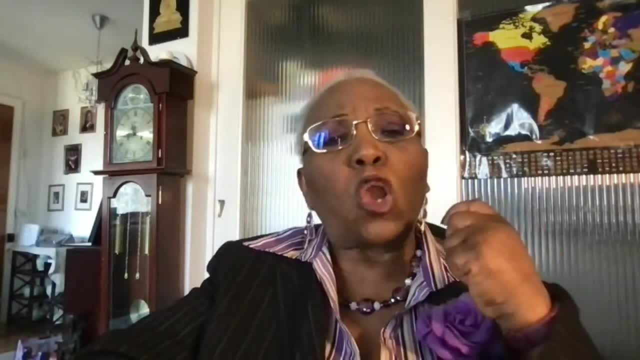 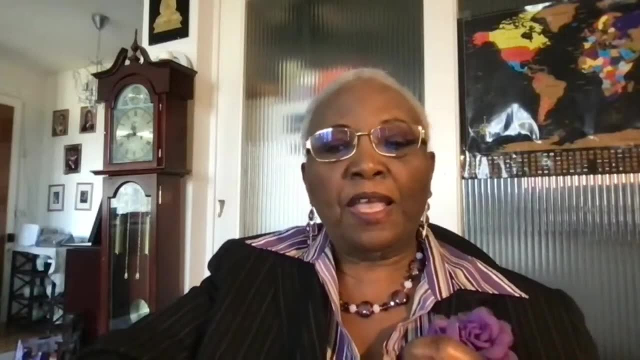 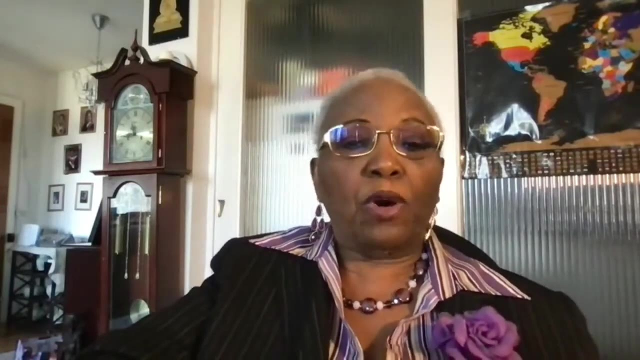 And it was only in 2015,, after years of lobbying and persuasion, that recognition was given to energy in the 2030 Sustainable Development Agenda. Indeed sustainable development goal is ensure access to affordable, reliable, sustainable and modern energy for all, With one of the targets as having universal access. 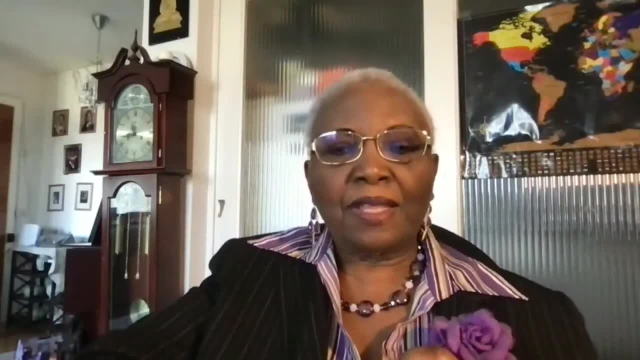 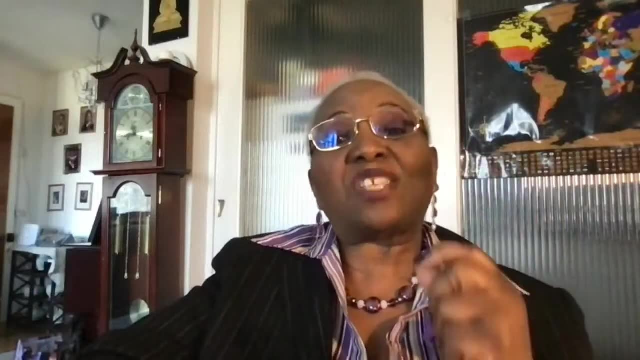 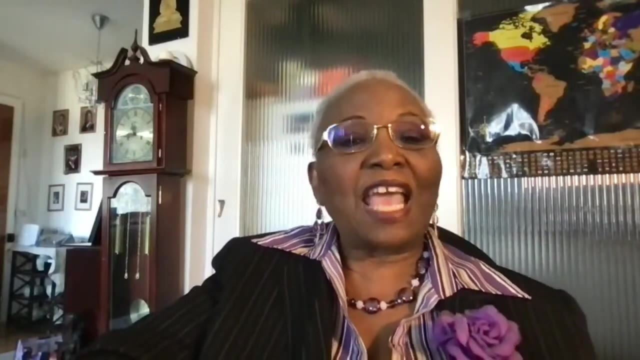 to electricity by 2030.. However, this is a target And, according to the UN, at the current rate of progress, it projected 620 million people would still lack access to electricity in 2030.. This estimate does not even take into account the disruptions caused by COVID. 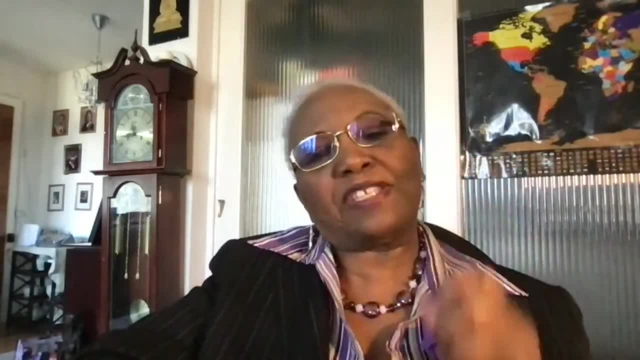 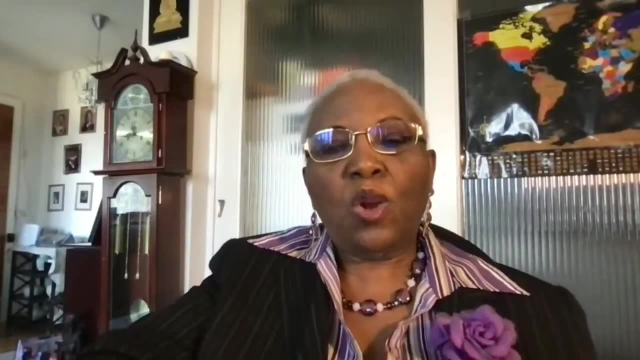 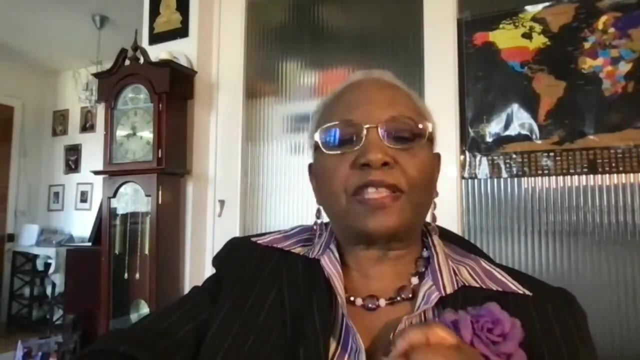 Yes, 620 million people, mainly in developing countries in general and Sub-Saharan Africa in particular, will have their human rights continue to be abused due to lack of access to electricity. The 2030 Sustainable Development Agenda: the UN's Sustainable Development Goals. 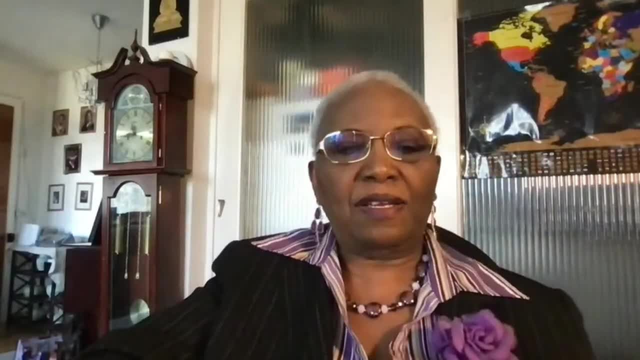 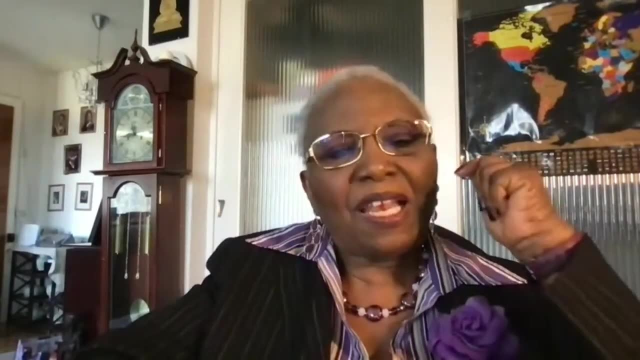 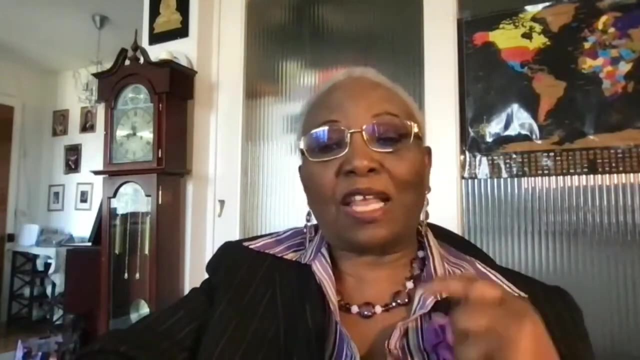 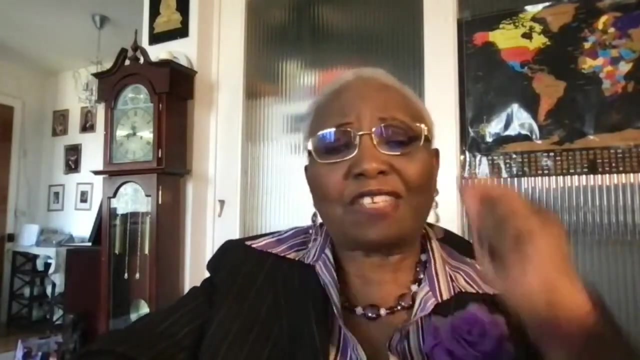 promise that no one should be left behind, But, as the facts show, Sub-Saharan Africa will be left behind or risk being left even further behind, in a world in which technological advancements make access to electricity indispensable for progress, Even in developed countries. recent events have demonstrated.